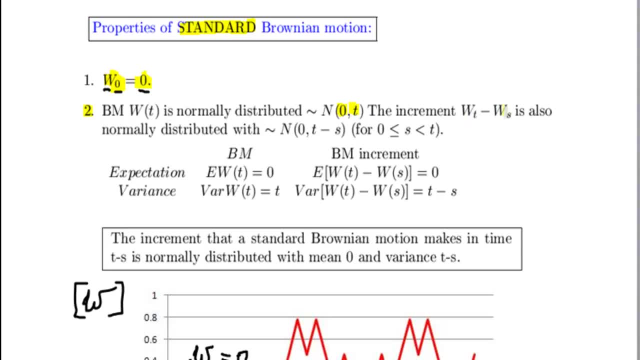 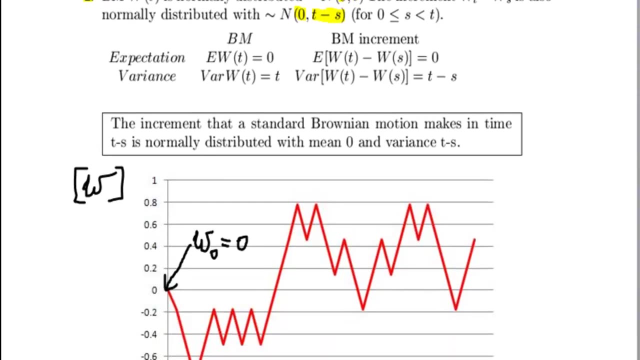 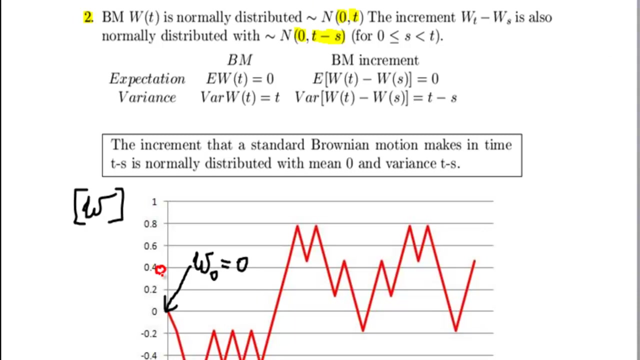 and Brownian motion increment W t – W? s is also normally distributed with mean 0,, 0 and variance t minus s. Okay, so what does it mean? that the Brownian motion is normally distributed with mean 0 and variance t, So say I'm standing here at time- equals 0, and 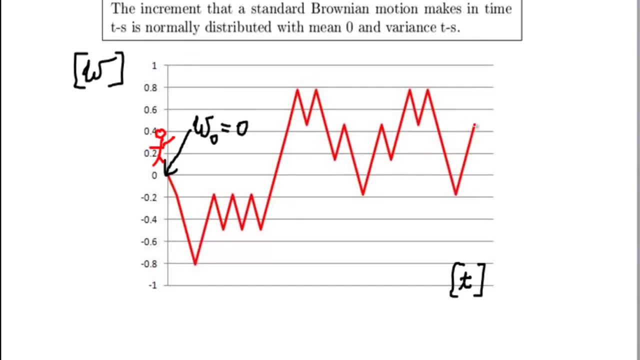 I want to know what my Brownian motion is or will be at time. say: time equals t equals 2.. Okay, so I see here that this single realization of Brownian motion happened to take a value of 0.4.. Okay, but this is just one realization. On the other realization, Brownian motion, 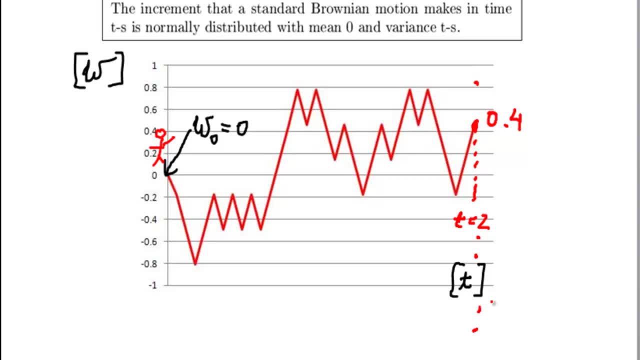 can end up here, here, there, there, there. It can pretty much end up all over the shop. ie, it can take a range of values. The good news, however, is that I will know what the expected value is. 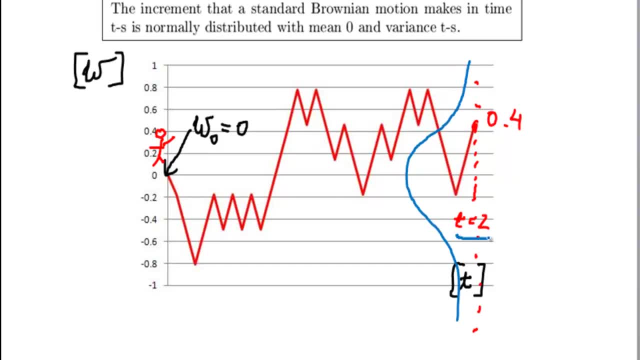 Okay, so this is the distribution of Brownian motion at time equals 2.. Okay, but the good news, I will know what the center of the distribution is, ie what the expected value of this distribution is, and this will be expected value of w at time 2 equals 0.. Okay, it will always be 0. 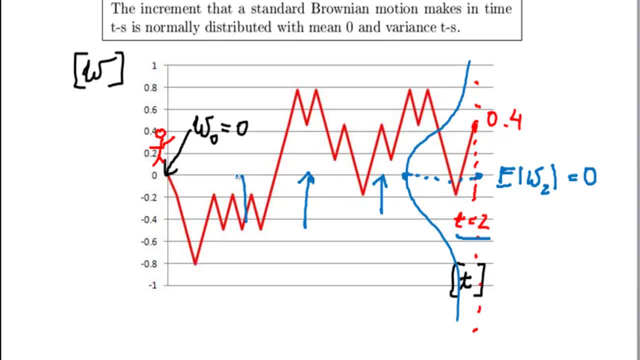 Whether I look at the Brownian motion here, here or here, the expectation of Brownian motion at all these points will be 0.. Okay, so this is the distribution of Brownian motion at all these points is 0.. So not only the mean or our expected value. that the value. 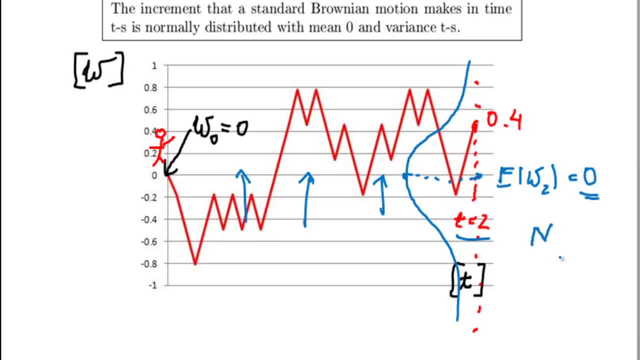 of the Brownian motion at any time will be 0,, but also we are told that it will be normally distributed. That's why here I graphed like a normal distribution. Okay, the peak of this distribution is centered at 0,, meaning that my Brownian motion will be distributed as 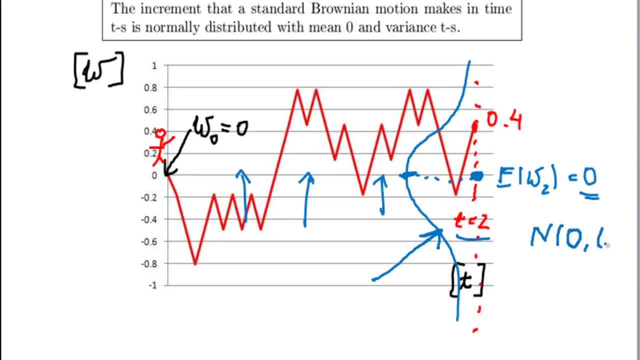 a normal variable with expected value 0 and variance t. Okay, now, crucially, it says t here. What does it mean? Well, if I look at the distribution of my Brownian motion, say, at this point here, then I will see that this distribution is also centered at 0, but the 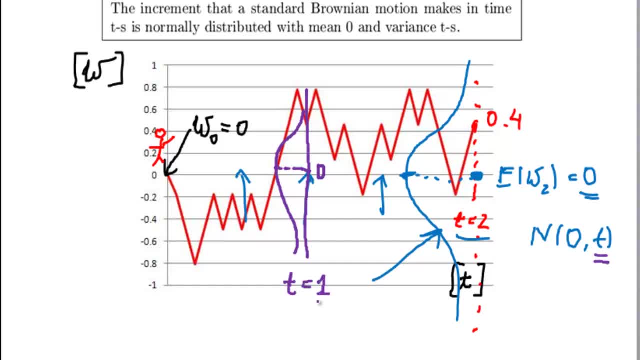 variance of this distribution, say at time equals t equals 1, is 1.. Okay, now the variance of this distribution- Brownian motion- at this point will be 2.. Okay, so my variance will basically so, if I have here, I will have t equals 1, and I will have t equals 1, and 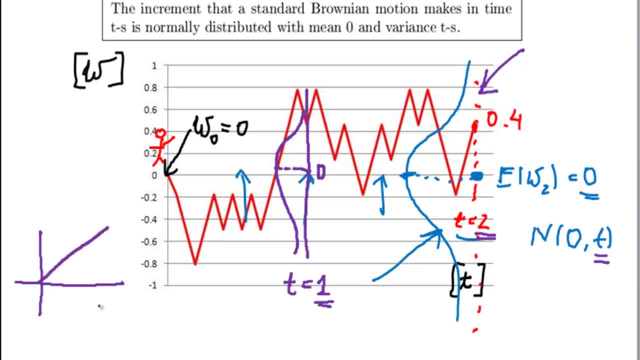 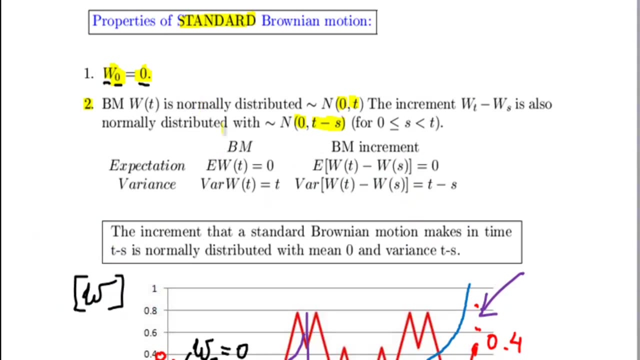 here. just draw another graph. my variance will increase proportionally to time. So this is variance I will denote here. sigma squared is proportional. is of order t. Okay, I think I've already spent too much time on this to illustrate such a simple concept. I only spoke. 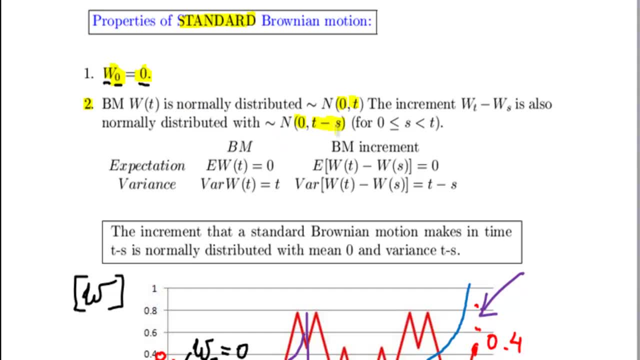 about Wt, but there is a related concept, ie the Brownian motion increment, which is the difference between two Brownian motions. okay, So one at time t, the other one at time t, the other one at time s, And it turns out that the difference between the two Brownian 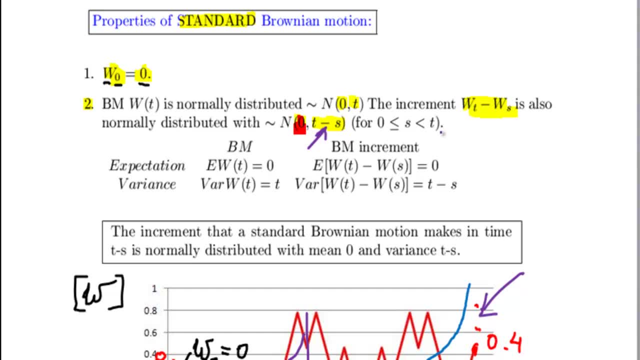 motions is also normally distributed and the variance of the Brownian motion increments, ie the difference between two Brownian motions, is just t minus s. t stands for time and s stands for time. It's just the difference in time between the measurements of our Brownian. 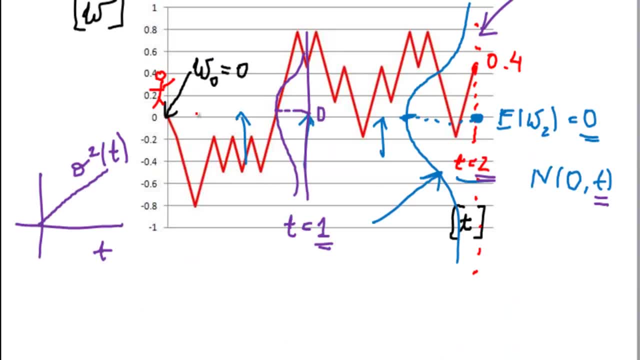 motions. Okay, so what this means if I look at my Brownian motion, somewhere at this point here and somewhere at this point here. so the expected increment, so this is time t, this is time s. the expectation of the difference of these two Brownian motions, Vt minus Vs equals. 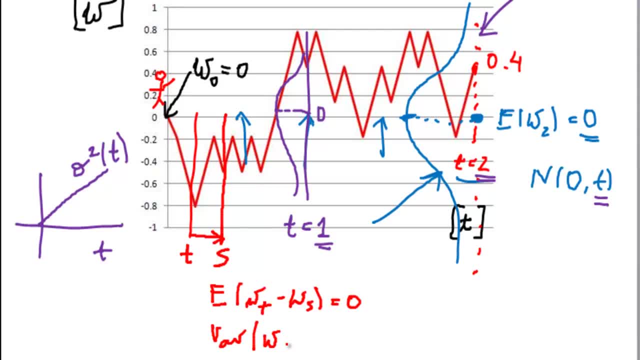 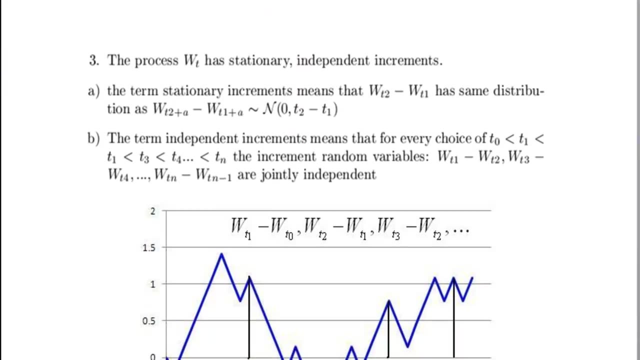 0.. And the variance of this difference equals t minus s. Yet again, it's proportional. variance is proportional to time. yeah, We'll show these properties more formally later on, but let's continue. let's discuss other properties of Brownian motion. 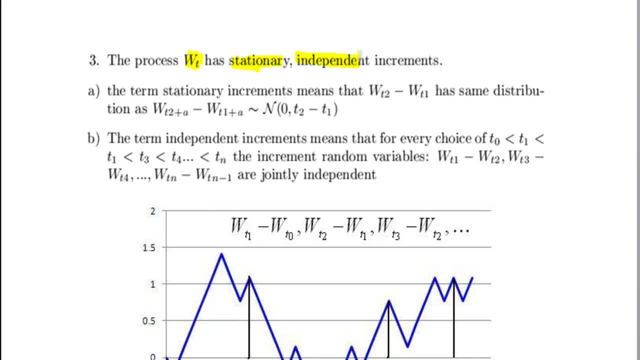 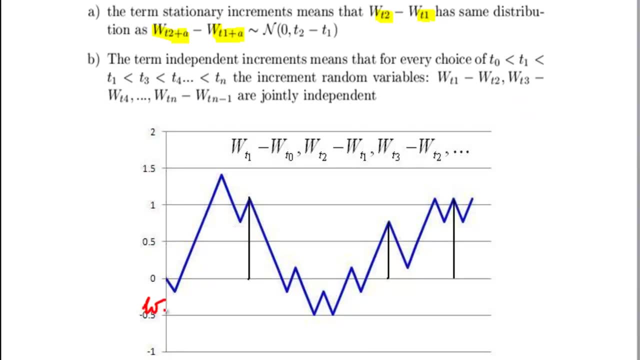 The process Wt has stationary and independent increments. Okay, so what does it mean that the Brownian motion has stationary increments? Well, if I look at my Brownian motion at time 0, and say my Brownian motion at time 1, and then I looked at my displaced Brownian motion, 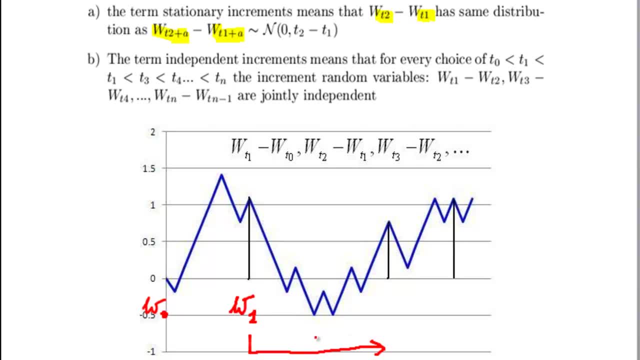 I moved the Brownian motion increment further in time by a constant of time, so that this a, So this is going to be to w0 plus a and w1 plus a, And what this means is that the distribution of this increment here will be exactly the same as the distribution of this. 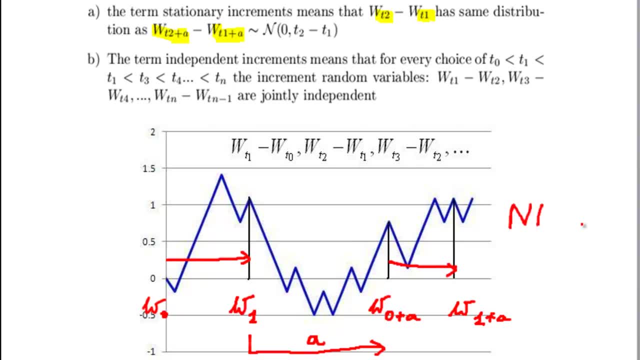 increment here. ie they will both be normal, with expected value of 0 and a variance of t1 minus t0. So it doesn't matter where you look at the Brownian motion, it will always have the same properties. okay, It's expectation. so we're talking here about the increments. 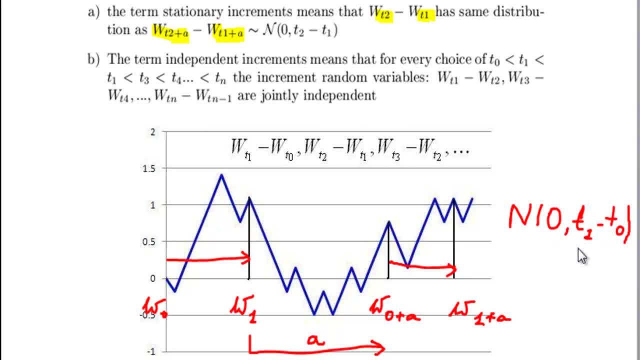 The incremental expectation will be always 0 and the variance will be just the difference in time. So to sum up, independently where you look at the Brownian motion, whether you look at Brownian motion here in this time interval or here, it will always have the 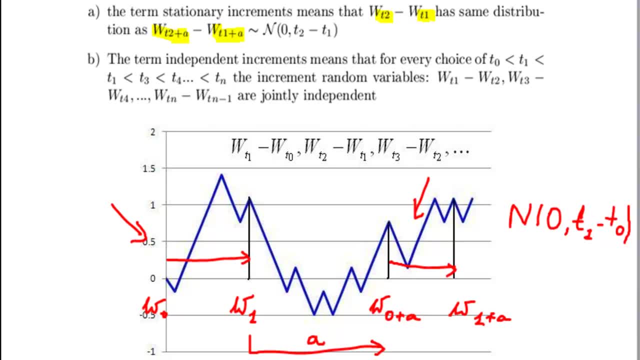 same properties In probabilistic sense. okay, we always have an expectation of 0 and variance will be proportional to time. Another property is that increments say w1 less w0 and w1 plus a less w0 plus a. what independence says is that whatever, however, I moved in this time interval will. 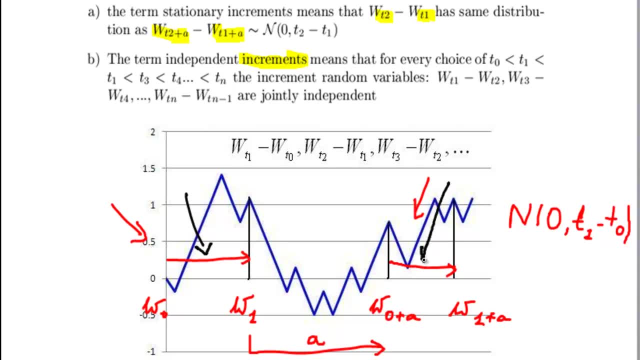 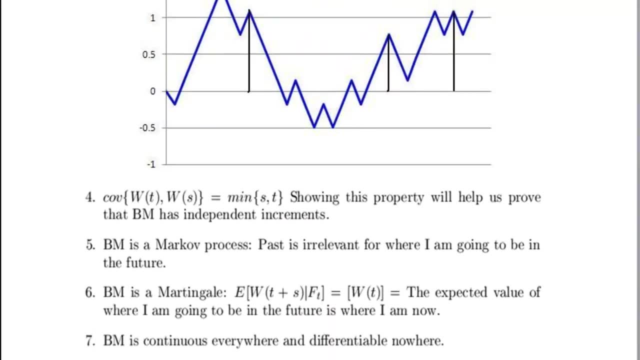 have absolutely no bearing on how I'm going to move in this time interval. Okay, I'm going to clear This graph. Let's see some other properties of Brownian motion. We'll briefly enumerate them without actually proving them at this stage. Covariance of two Brownian motion paths. 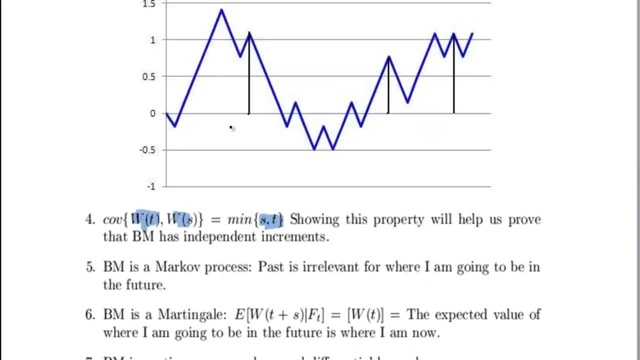 is the minimum of time s or t. So say, I look at my Brownian motion at time s and I look at my Brownian motion at time t And if I try to find covariance of these two terms, I will find that the covariance will be the minimum. 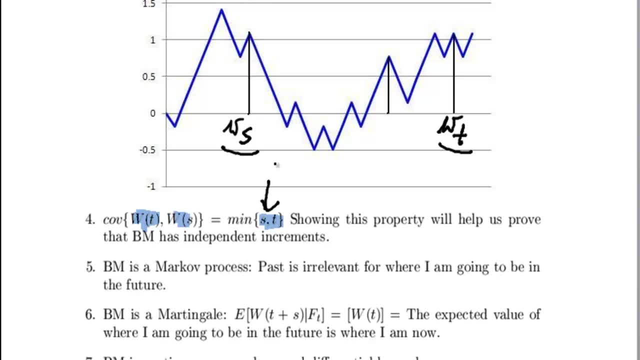 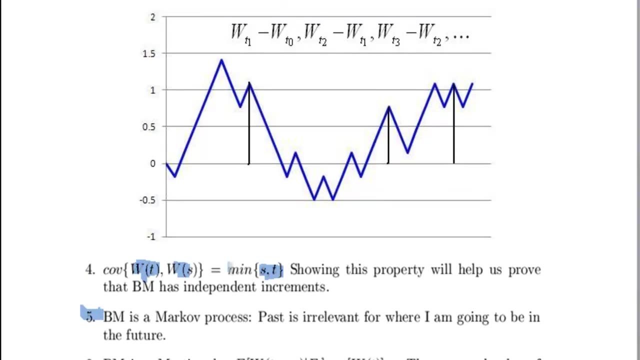 The fairness of s and t, When here it's clear that s is before t. therefore, the covariance of these two terms will be s Property. number 5, says Brownian motion, is the Markov Process. Okay, what does this mean? Markov Process? All it means is that past is irrelevant from 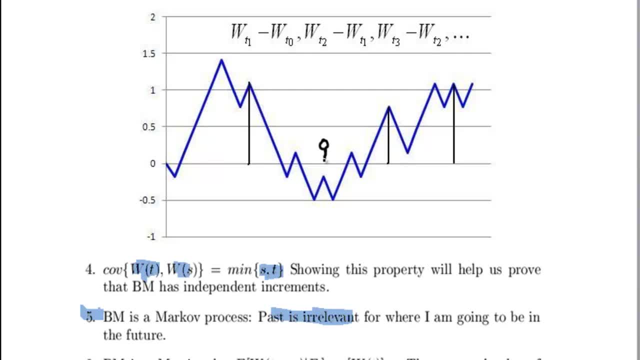 where I'm going to be in the future, Say: we are here, so I'm here. at this point It's irrelevant what I've done in the past. It's irrelevant how I moved in the past for where I'm going to be in the future. So past has absolutely no bearing on my future evolution. 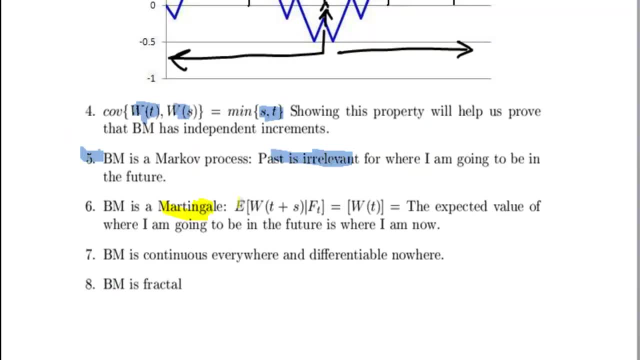 Next property, Brownian motion is a martingale. Okay, so this says expected value of Brownian motion, which moved by time s. So I'm at time t and it moved by time s. Conditional or all the information. conditional filtration, ie all the information I have available at time. 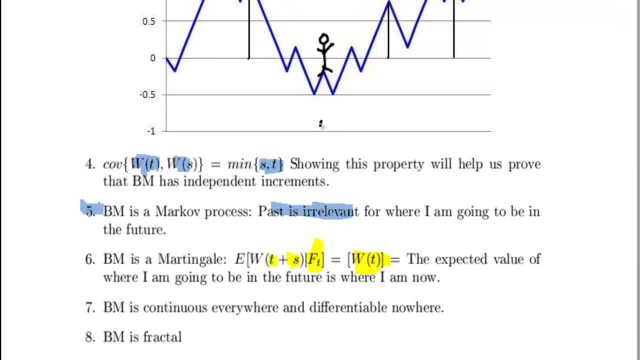 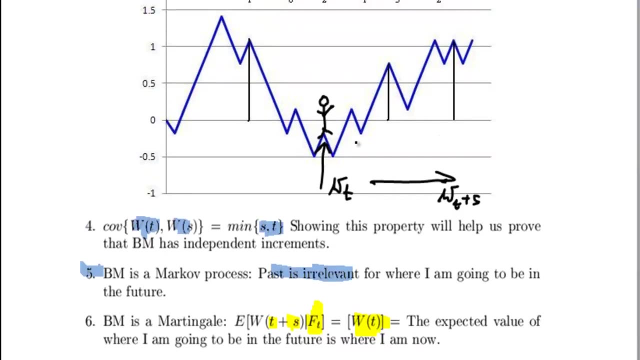 t is just where I am at the moment. So yet again, this martingale property can be illustrated. Imagine that I'm standing here at time wt. I ask myself a question where I'm going to be at time wt plus s? Well, according to the martingale property of Brownian motion, my 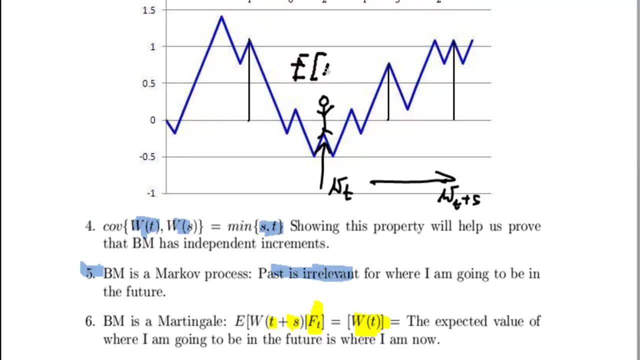 expectation of where I'm going to be at time. dt plus s. Conditional on all the information I have. how I moved in the past. Okay, here I move up, down, up and down several times. Conditional on all the information I have, what I've done. 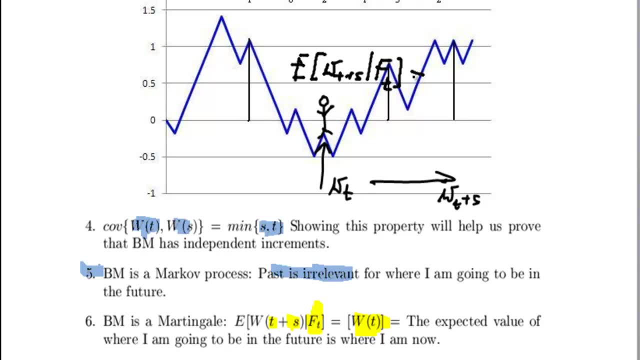 in the past, which is denoted by F capital T is nothing else but wt. Okay, so what this means is that I don't expect to have moved at all. I expect to stay at the same level, ie somewhere here. so negative, Okay, I expect to be at the same point at time. t. 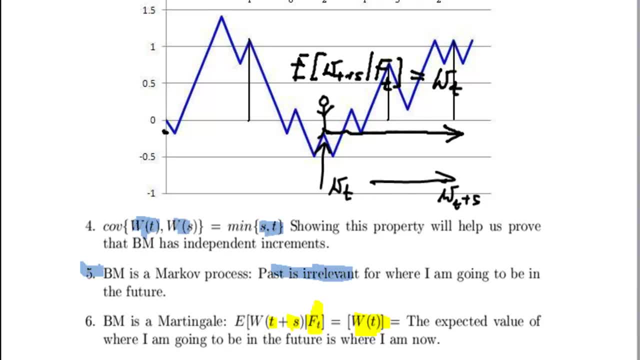 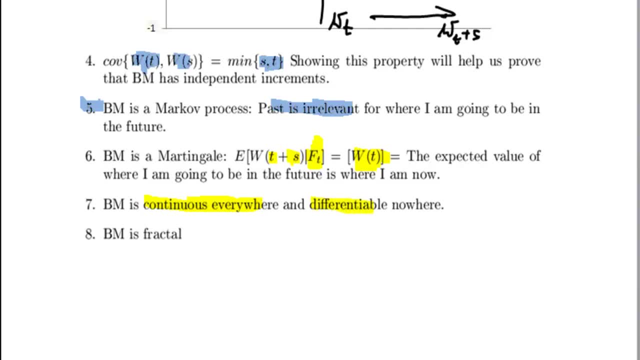 plus s, as when I was at time wt. Finally, Brownian motion is continuous everywhere. This is property number seven and differentiable nowhere. What this means is that you can probably see it here: It's continuous everywhere because there are no jumps, there are no discrete. 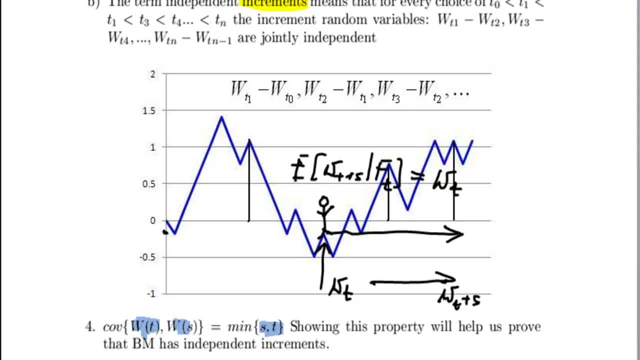 continuities in this Brownian motion and you cannot differentiate it anywhere. Okay, so let me erase one more time the chart Hold on. you may ask: Well, surely this for instance. let's have a look at this bit. Okay, so let me erase one more time the chart Hold on. you may ask: Well, surely this, for instance: let's have a look at this bit, Okay, so, let's have a look at this bit, Okay so, let's have a look at this bit, Okay, so, at any point,